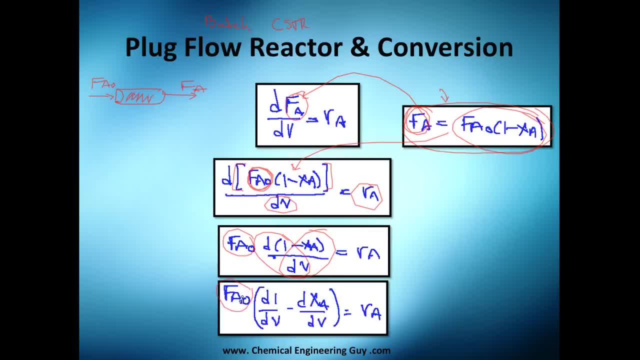 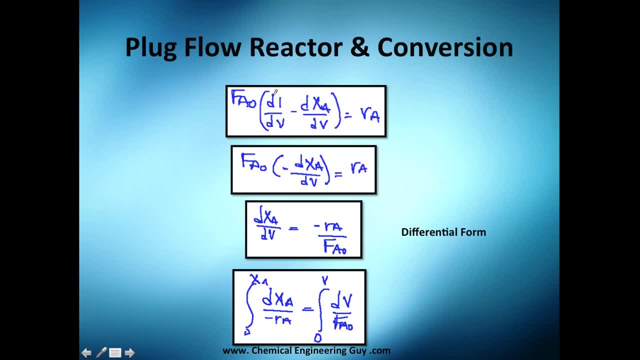 respect of volume. Everything I just said multiplies my flow and the right side stays exactly the same. Now, by mathematics, hopefully, you know that the derivative of any constant is 0, so this is 0, it goes away And I'm left with the flow which multiplies this value. here The thing is, I love having differentials. 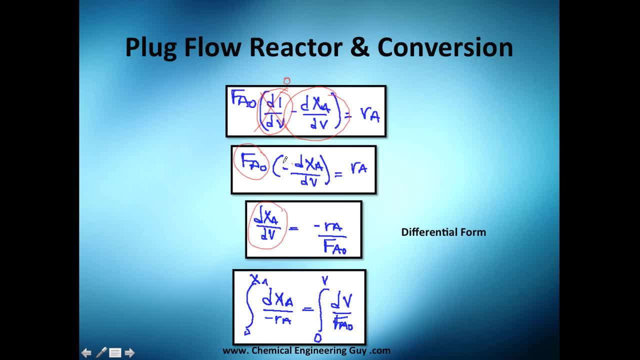 or derivatives. so I'm going to get this derivative value. I take away this negative sign and this flow. so I pass this dividing and this negative. I pass it to the right. As you can see, I am a great fan of this rate of reaction concept. If you don't have the negative, then it's not the rate of reaction. 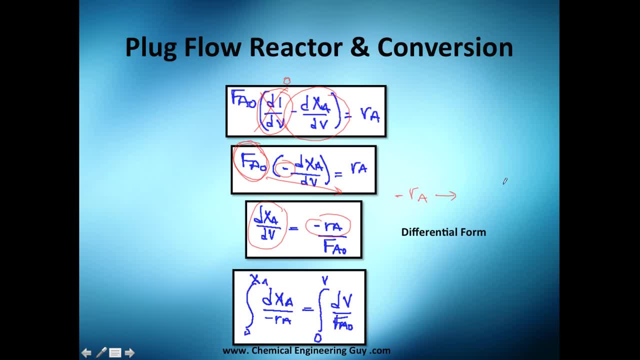 it's actually a rate concept of production, so you're going to get used to actually use the rate of reaction. be sure to add that negative sign. now, that's the differential form. as i told you before in the batch video, many persons love the integral form, which means they have already integrated. so let's go and integrate. 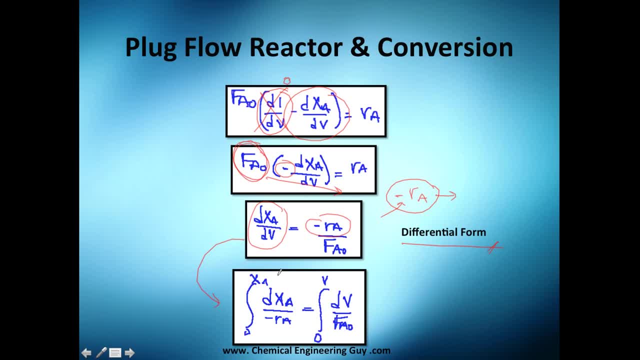 it left side, we leave this differential of conversion. once again, this rate of reaction is dependent on that. so we differentiate from zero to x or conversion. then we send the differential here to the right. that's a differential of volume divided by this. you can take it out. 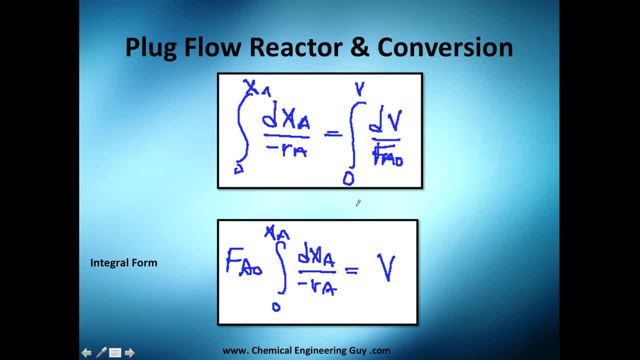 because it's a constant, and i think that's what we're going to do. yes, look how the version is directly dependent on the volume. you start from zero and the higher the conversion, the higher the volume and backwards. so what i want to do is essentially get this here and integrate. 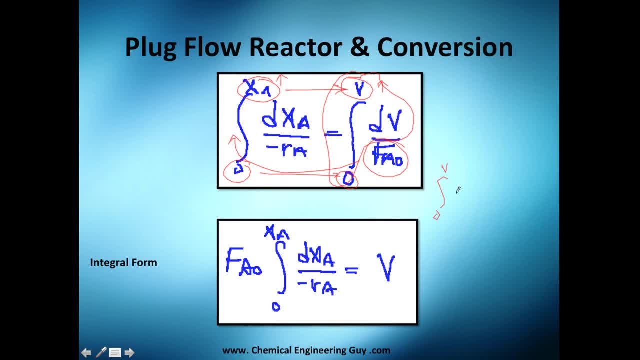 this integral, which you know, it is the integral of zero to b, from d: b. this is one, but you need to evaluate it in zero and b. sorry, one b b minus zero, you get b. so that's why i get this volume and yeah, essentially we're done. guys, this is our integral form, actually.